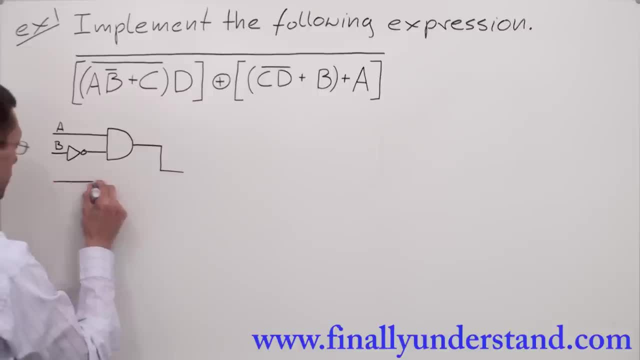 of the parenthesis. This is going to be my C North with D And gate. Next, the whole term inside of the parenthesis is ANDed with D, So I'm going to have D over here. Next, the whole term inside of the parenthesis is ANDed with D. 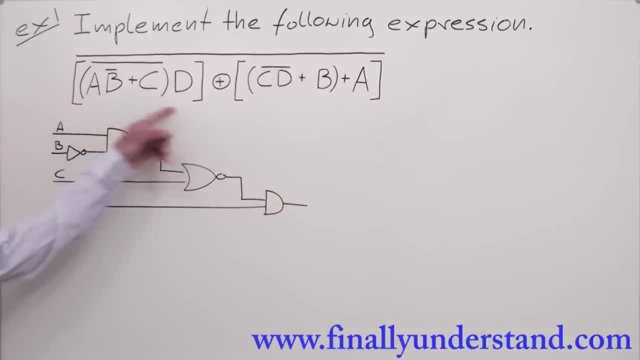 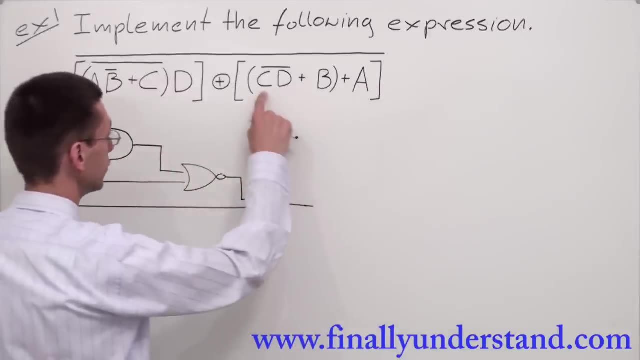 So I'm going to have D over here. We're finished with the very first brackets. Let's take a look at the second part of our expression. Inside of the parenthesis, we have AND gate with two inputs. I have input C And I have input D. 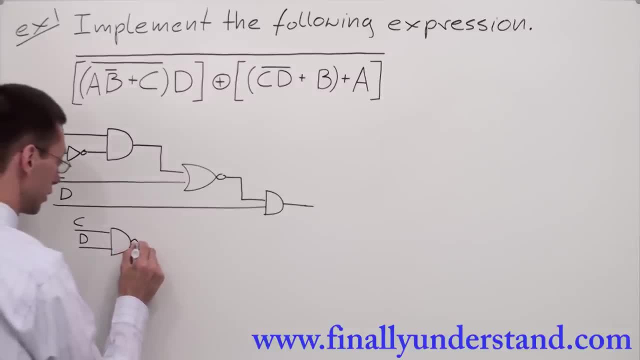 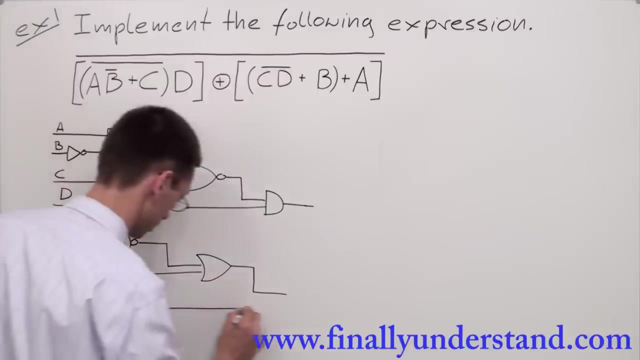 This AND gate is a- C. I have input D, So I'm going to have D over here. nut gate is ORed with input B, So this is my OR gate. The whole term inside of the brackets is ORed with A, So I have to draw another A input and this is ORed together. 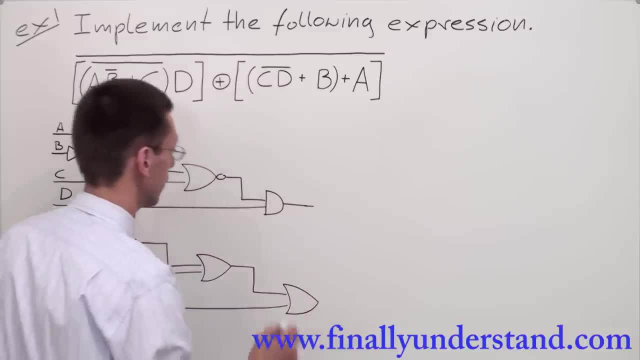 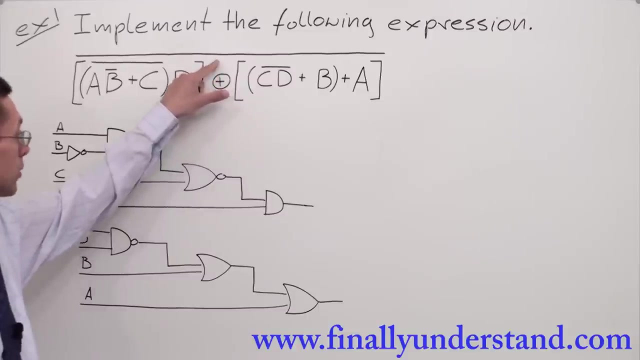 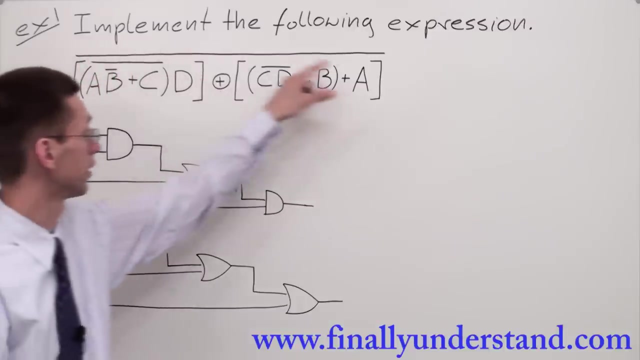 with the parentheses. Now, if you are going to look at our original expression, you will notice that these two circuits are exclusive NOR together. Why? Because this symbol stands for exclusive OR and because we have the bar over that sign means this is exclusive NOR. We have to connect. 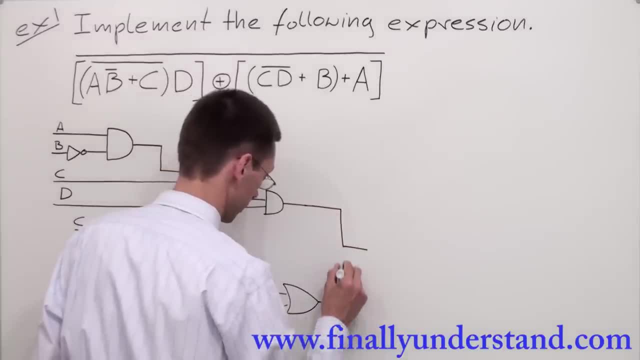 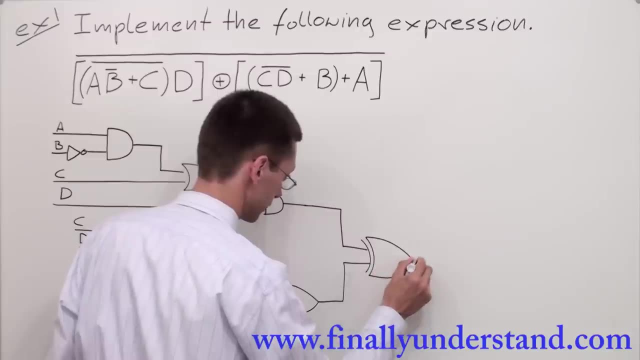 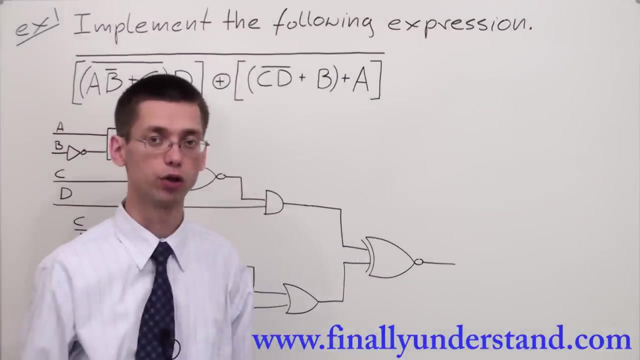 these two circuits by the exclusive NOR gate? Yes, This is my answer. Right now I'm going to perform the analysis of this circuit and I'll try to prove that my circuit is going to give me exactly the same Boolean expression. Let's take a look. We have A going to the input of the AND gate. We have B going to 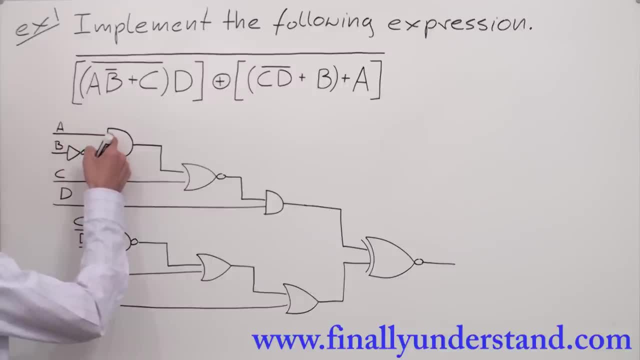 the input of the AND gate. This is exclusive N. this is close to the paisent victims. This will give me the exact connect. The other one is 352B. So what does it mean? This is just the 넿 gate. 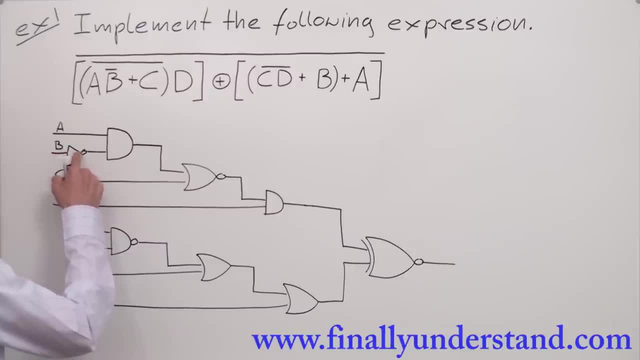 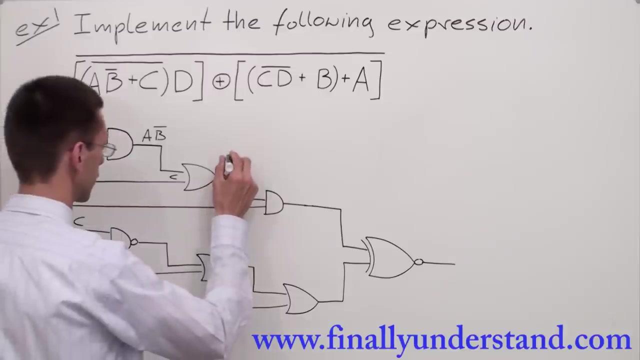 b input connected to the inverter. and on the output of the inverter, i'm going to have b naught. a times b naught will give me a b naught, c, c will go to the second input of my nor gate. on the output of the nor gate, i'm going to have a. 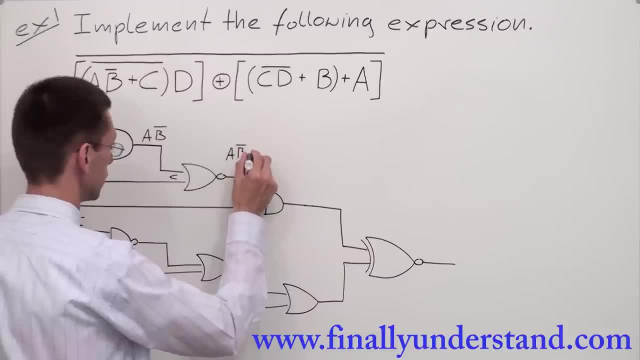 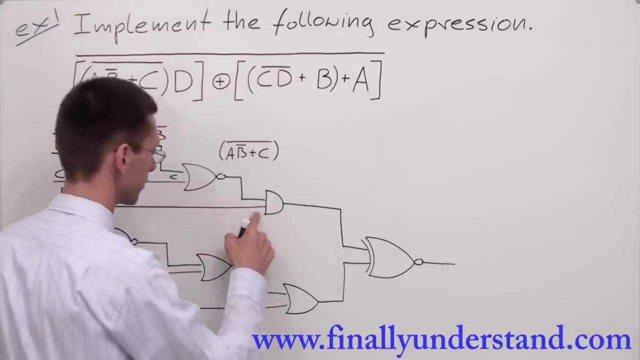 b, naught, nor c. i can put this inside of the parenthesis now. next, i have the input connected to the end gate. so it means whatever is on the first input has to be multiplied by the second input. so it means that i'm going to have a- b. 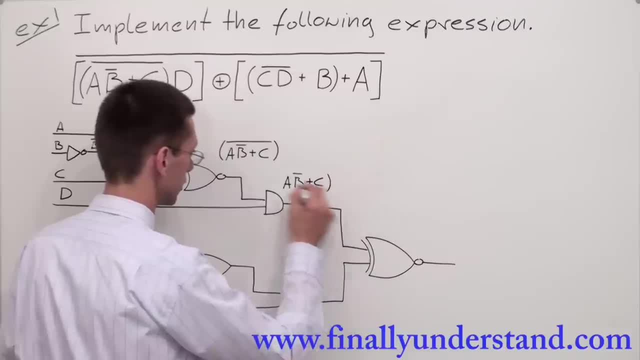 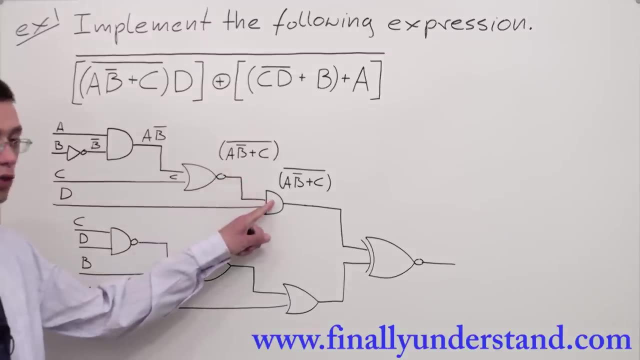 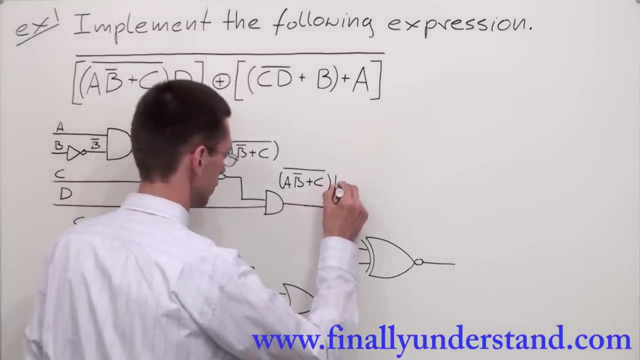 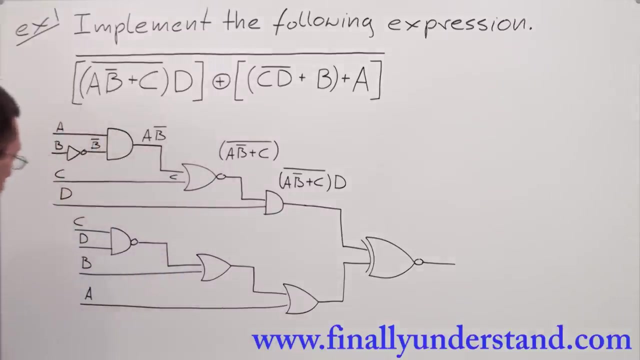 not plus c, not. this is the expression which goes to my first input of the end gate and we have to multiply this to d, remember, and gate stands for the multiplication. now let's check the second part of the circuit. i have c and d on the inputs of non-gate. 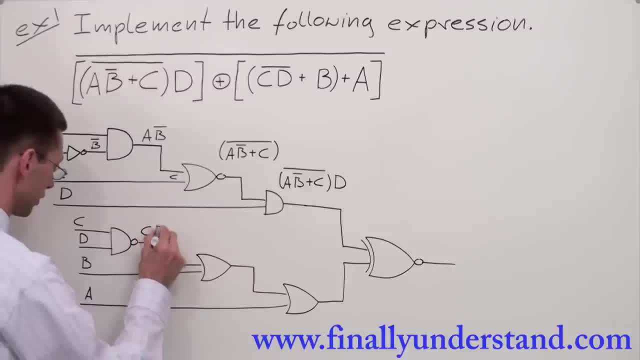 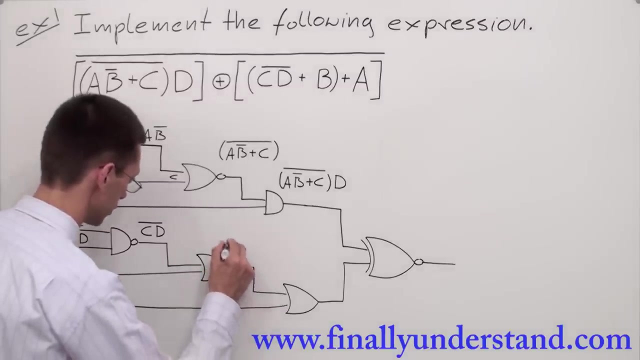 so, on the output, i'm going to have c, d, remember this is multiplication. but because i have bubble over here, i'm going to have bar over these two variables, over the product of these two variables. next, this expression will go to the or gate another. the OR gate has B, So means I have to see D node, OR with B, A input goes to my. 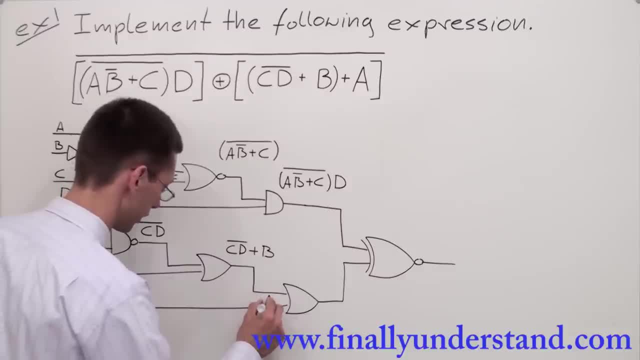 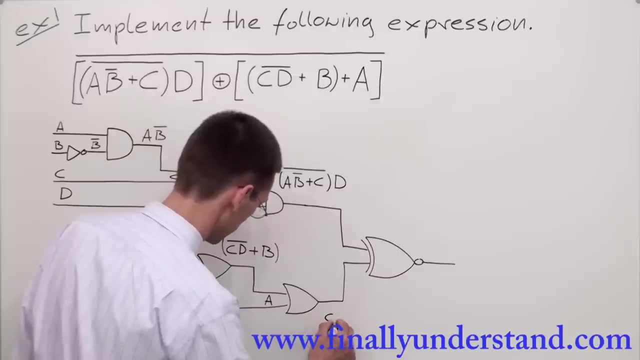 other OR gate and this is going to be my A and this expression will go to the first input and A will go to the second. Remember this is my addition. so I have C, D node OR B. We have to OR it this with A.